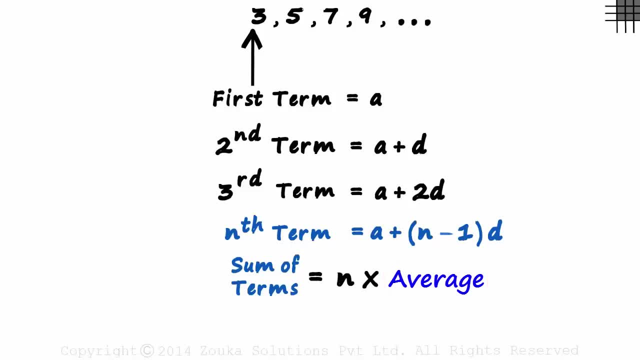 Understanding the average is the best part of it. All sequences are evenly spaced numbers. For evenly spaced numbers, the average is the sum of first term and the last term over 2. That's it. We get the sum of terms if we know the number of terms. 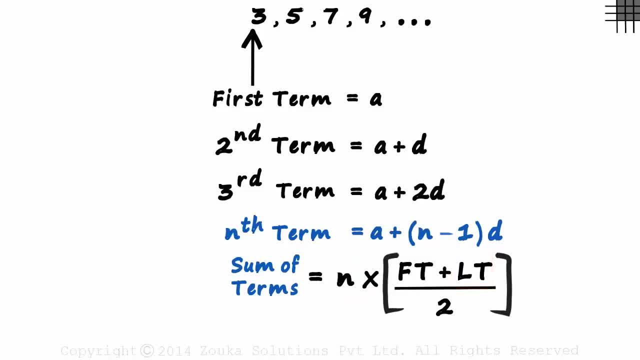 the first term and the last term. The sum of terms in a sequence is called terms. It is called series. We will understand more about it in our future sessions. Let's take the two outside and write n by 2.. The first term is a and this is the last term. 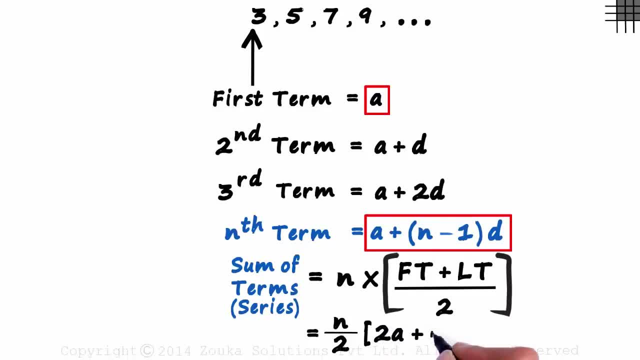 So first term plus the last term is equal to 2a plus n minus 1 times d. This is the formula to find the sum of terms in a sequence. But wait, This is only an arithmetic sequence. Yes, This is an arithmetic sequence, as the difference between two consecutive terms is constant. 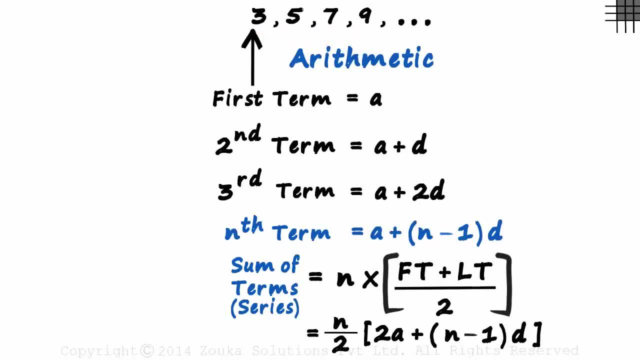 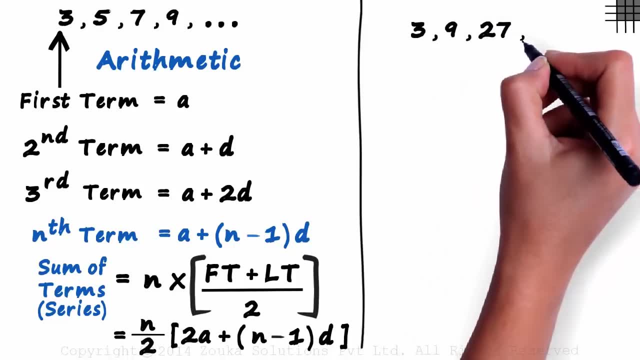 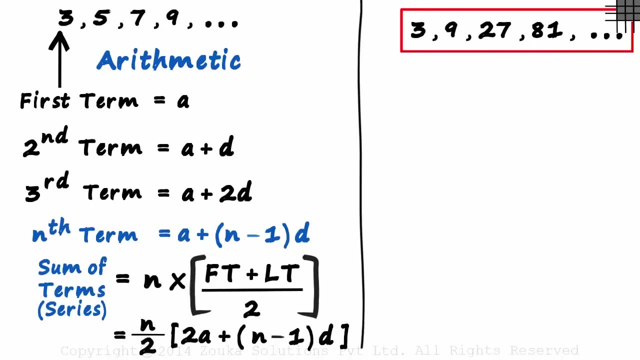 But wait, What are the other types of sequences? then, To look at more types, we go through the next sequence, 3,, 9,, 27,, 81 and so on. Pause the video and think about whether this is a sequence or not. 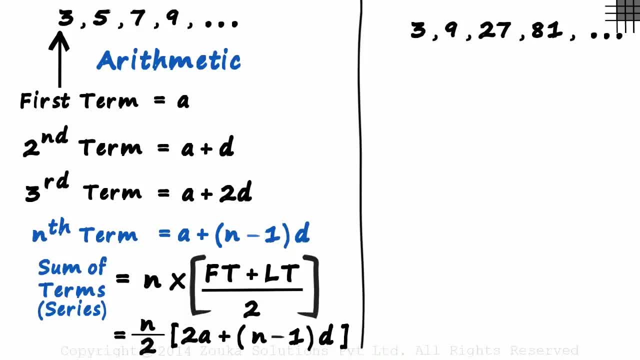 OK, Some of you would have assumed that, as the difference between two consecutive terms is not constant, this is probably not a sequence. Don't forget the definition of a sequence. It is simply a set of numbers which have some pattern, And the pattern can be anything. 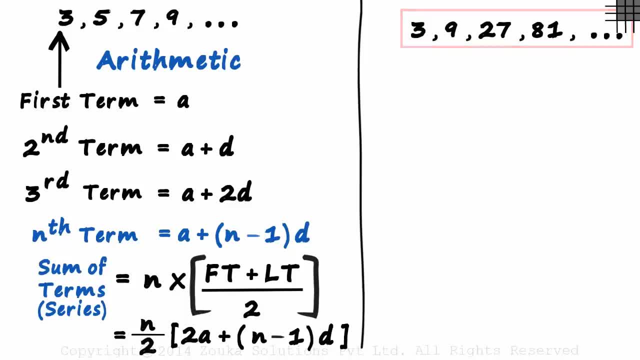 Did you spot a pattern here? Look at the ratio of two consecutive terms. The ratio 9 over 3 is equal to 3.. And the ratio of 27 to 9 is also 3.. Just like the common difference in arithmetic, we have a common ratio here. 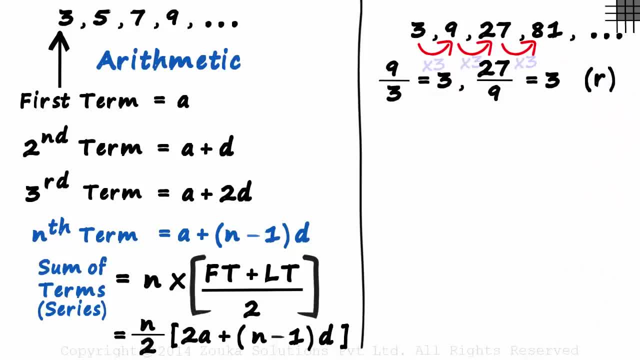 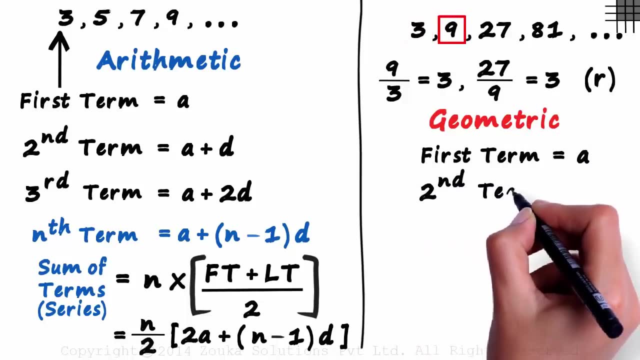 We can call it r. Each term is multiplied by 3 to get the next term. This is called a geometric sequence or progression. Let's assume the first term of this sequence as a. What will be the second term then? It will be a times the common ratio r. 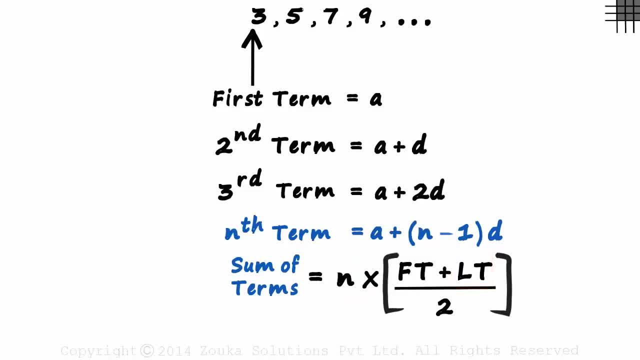 the first term and the last term. The sum of terms in a sequence is called terms. It is called series. We will understand more about it in our future sessions. Let's take the two outside and write n by 2.. The first term is a and this is the last term. 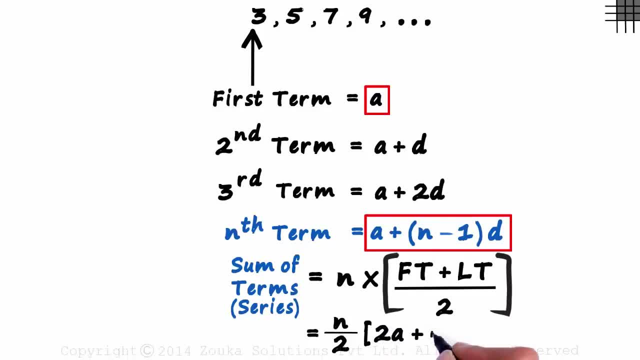 So first term plus the last term is equal to 2a plus n minus 1 times d. This is the formula to find the sum of terms in a sequence. But wait, This is only an arithmetic sequence. Yes, This is an arithmetic sequence, as the difference between two consecutive terms is constant. 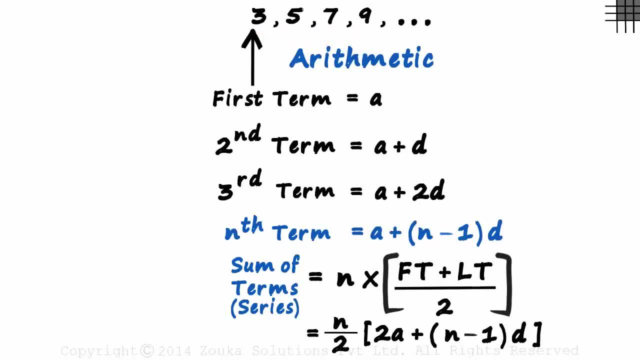 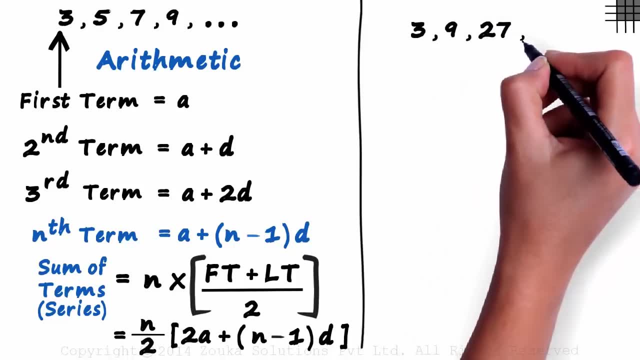 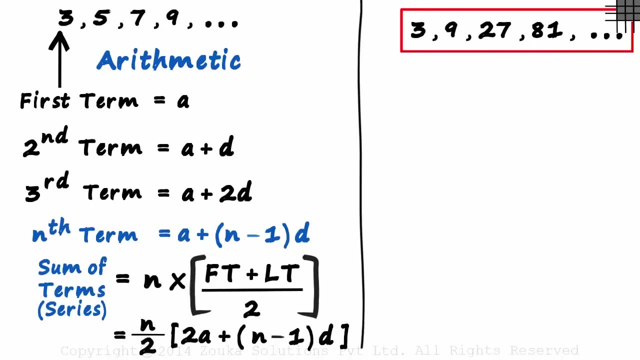 But wait, What are the other types of sequences? then, To look at more types, we go through the next sequence, 3,, 9,, 27,, 81 and so on. Pause the video and think about whether this is a sequence or not. 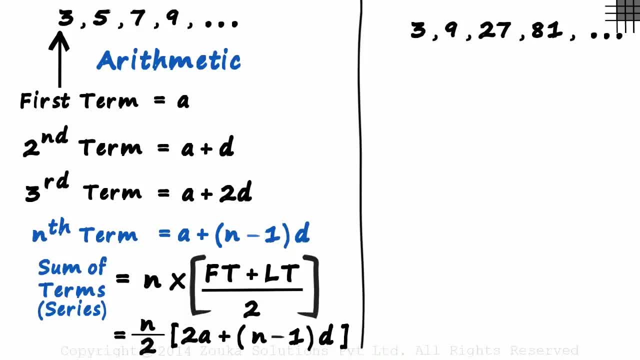 OK, Some of you would have assumed that, as the difference between two consecutive terms is not constant, this is probably not a sequence. Don't forget the definition of a sequence. It is simply a set of numbers which have some pattern, And the pattern can be anything. 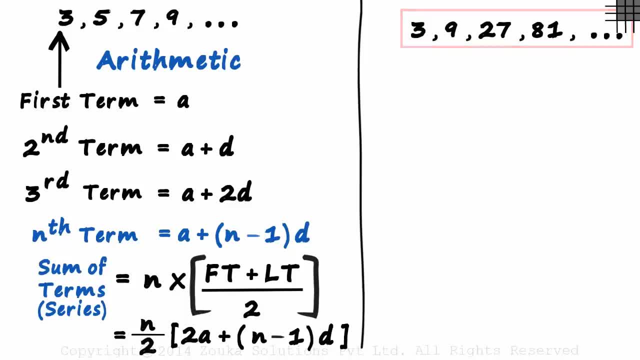 Did you spot a pattern here? Look at the ratio of two consecutive terms. The ratio 9 over 3 is equal to 3.. And the ratio of 27 to 9 is also 3.. Just like the common difference in arithmetic, we have a common ratio here. 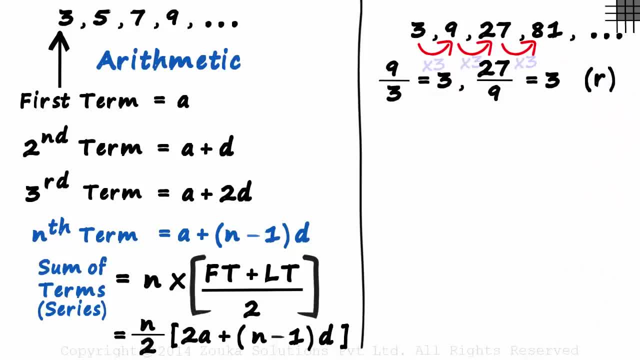 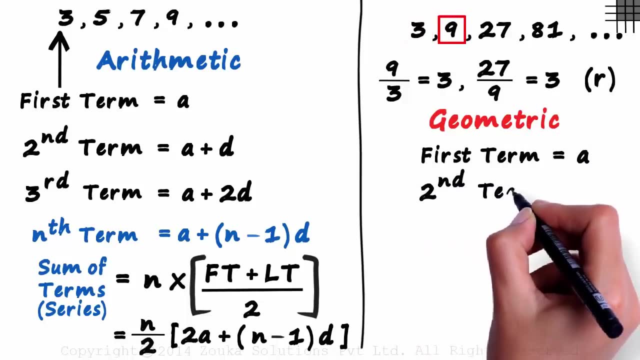 We can call it r. Each term is multiplied by 3 to get the next term. This is called a geometric sequence or progression. Let's assume the first term of this sequence as a. What will be the second term then? It will be a times the common ratio r. 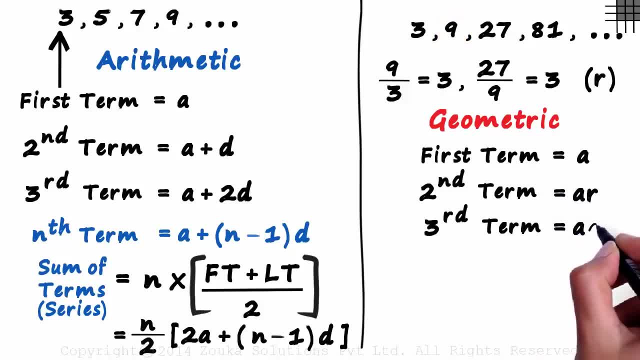 And the third term It will be a times r squared. And what will be the nth term of a geometric progression? Look at the pattern. Second term: r raised to 1.. Third term: r raised to 2.. So the nth term will be a times r raised to n minus 1..